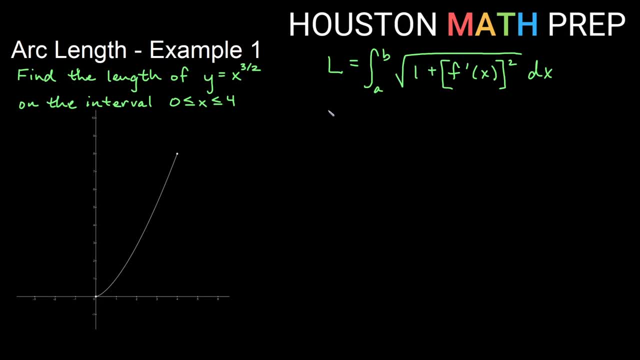 we're going to go ahead and do the steps. So we mentioned that the first thing you would do is to take your function and find its derivative. So our f of x here is x to the three halves in this example. So if I find the derivative of f of x, so f prime of x, this is just going to be a. 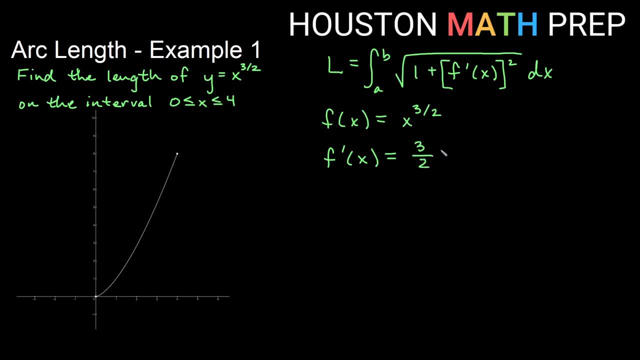 power rule. So the power comes out front, we get three halves, x to the. now the power goes down by one. so three halves minus one would be one half and x to the one half you might think of as if you prefer the square root of x. right, so that would be three halves. square root of x for f. prime of x. 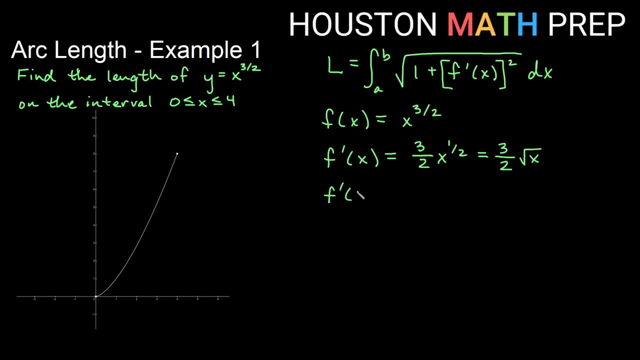 Now in the formula f prime is squared, so we go ahead and find f prime of x squared, so we'll square what we just got. So if I square the three halves I get nine on top, four on bottom, and then square root of that would be x, and so we have nine fourths x for our f prime squared. So I'll put: 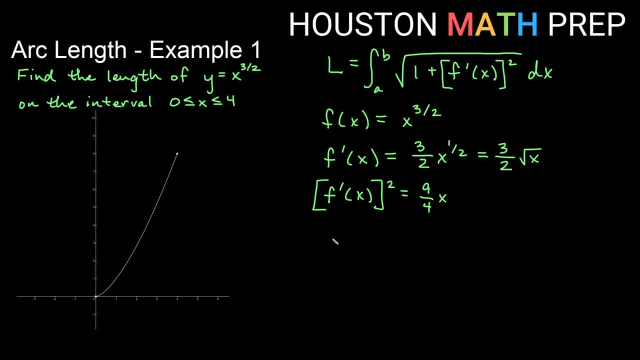 that in the root, I'll add one to it. let's go ahead and do that. so our length on this function, from x equals zero to x equals four, is going to be the integral one plus nine fourths x, square root of that dx. Okay, so this would require a. 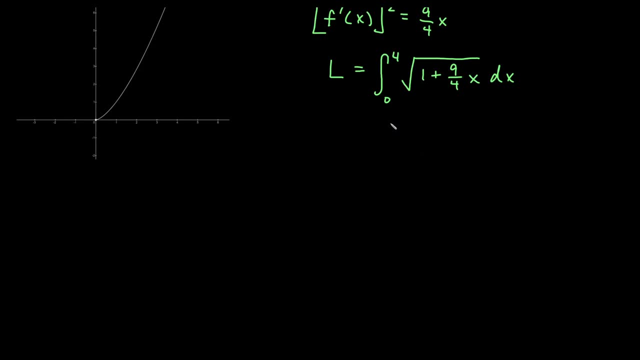 substitution. so I'm going to go ahead and do a u substitution here. So I will say that u equals what's inside of the square root, one plus nine fourths x, and if that's true, then du is equal to nine fourths dx. so in other words, 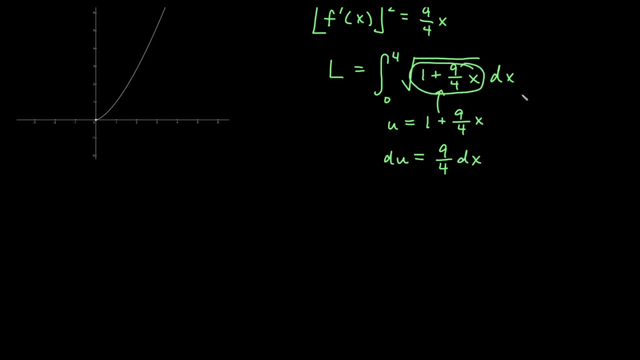 this part here is going to be u and then dx. if you're not sure how to sub for dx, we could go ahead and solve for dx. I could multiply by the reciprocal on both sides and get that four over nine du is equal to dx, So this part here would actually be four ninths du. 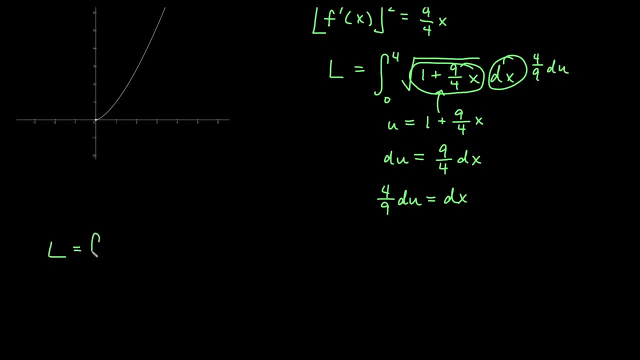 Okay, let's go ahead and work that, so we'll get that. the length is going to equal. now, remember, these are x bounds, not u bounds. so even though I'm changing into u, I'm going to go ahead and leave these as x bounds. so I would have the square root of u and then my dx becomes four. 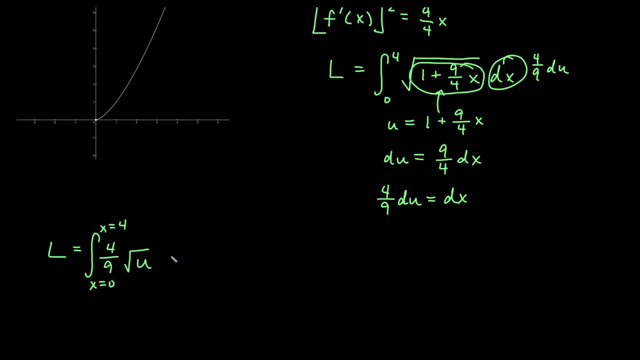 ninths du. so four ninths du. Now a couple of things. we can obviously bump the constant multiple out, so we can think four ninths times our integral. So four ninths again. remember these are x bounds from zero to four. and then, if you want to think of 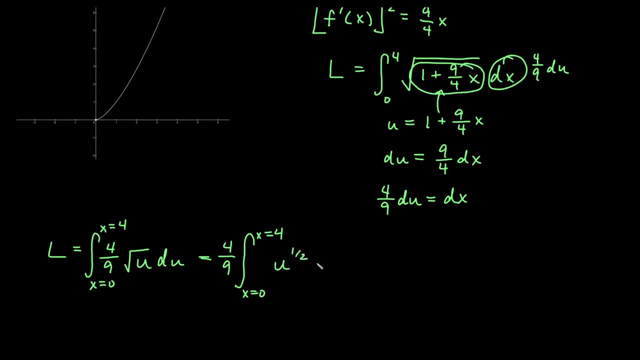 this as a power rule u to the one half- again that idea that square root is the one half power of something. So now I can do this as a power. so I keep my four ninths multiple and if I'm integrating this then my power will go up by one. so if I add one to a half that will be three halves. I will. 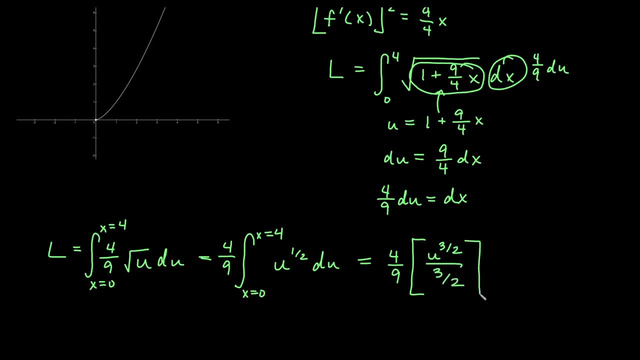 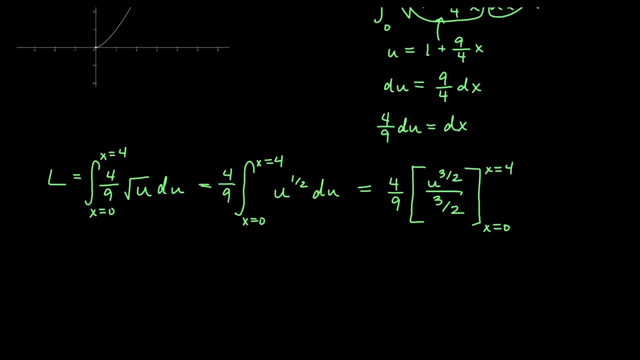 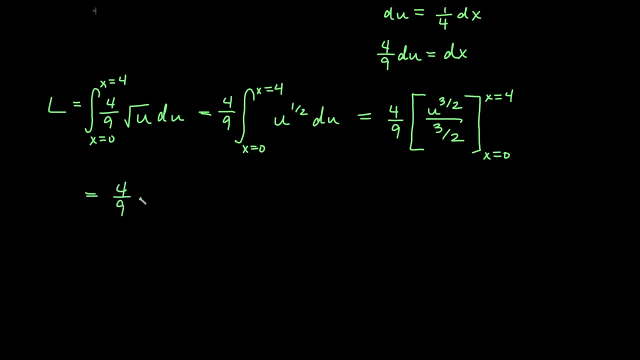 write that in. we won't leave it like that, for sure, right? so divide by that new power from x equals zero to x equals four. Now a couple of things. so divide by three halves is going to be the same as multiply by the reciprocal right, so you're really going to have four ninths times two thirds instead. 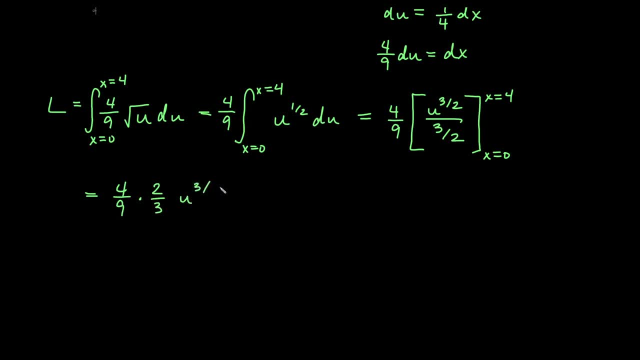 of divide by three halves- u to the three halves- and we will be evaluating that from x equals zero to x equals four. So I'm going to do a couple of things. I'm going to multiply my constants out here so I'll actually get eight over 27 in the front, and I'm going to go ahead and replace my u and if 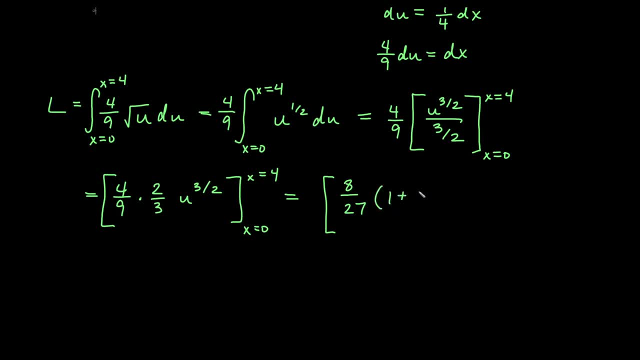 you remember u was one plus nine fourths x. so I will have that to the three halves and now that I'm back in terms of x, I can just rewrite the bounds as zero times two thirds. So I'm going to do a couple of things. I'm going to multiply my constants out here. 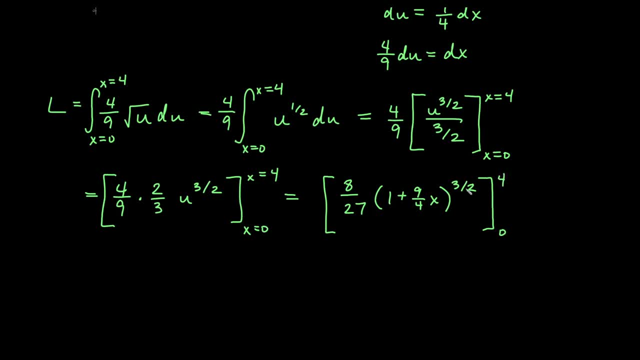 and not have to write the x equals. if I don't want to, I still can. So when we do this and we plug in, we'll have to remember three halves powers. so the bottom here means square root, the top means cubed right. so first thing we'll do is we'll go ahead and say eight over 27. I'm just going to bump that. 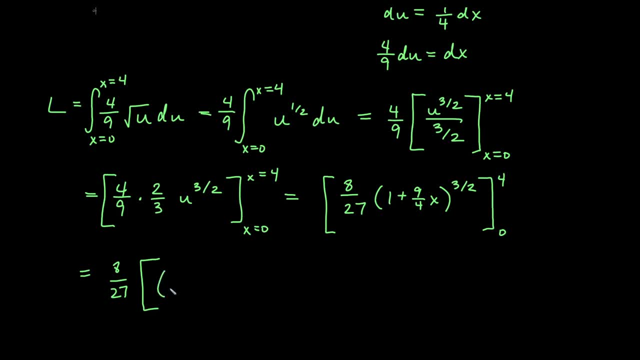 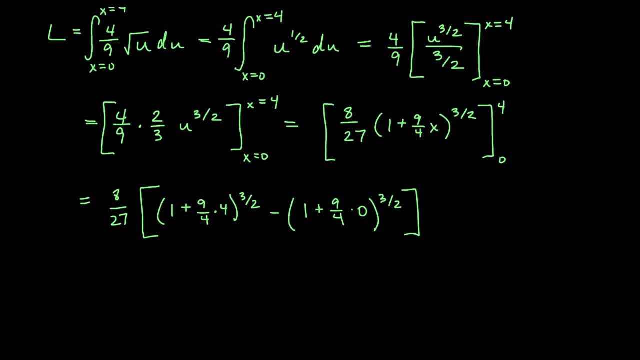 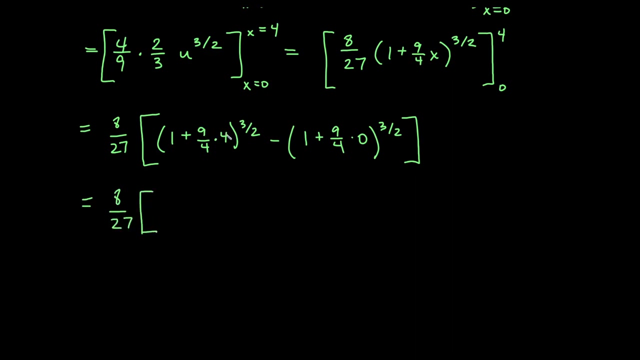 out. so if I plug in the four, then that will give me one plus nine over four times four to the three halves, minus one plus nine over four times zero to the three halves. Okay, and now we need to just do some arithmetic here, so we'll get eight over 27 here. the four is going to cancel with the four. 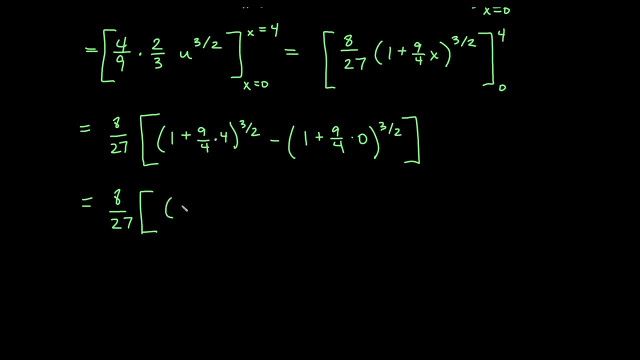 down there that becomes a one. so we get one plus nine, so we get 10 to the three halves minus, and then here this would become zero. so one plus zero would be one to the three halves. now anything, any power of one, is just going to be one, right. so this is really going to be eight. 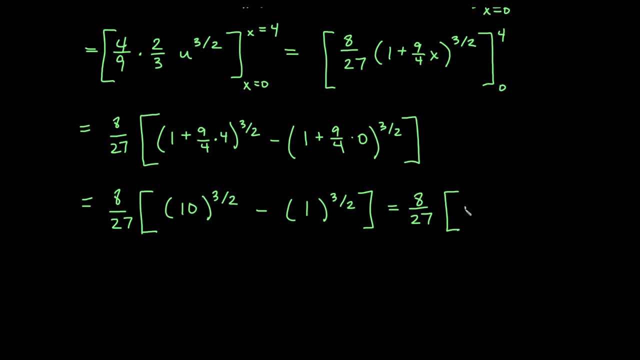 over 27, and then we'll have 10 to the three halves minus one. we could leave it that way in terms of units. Another way that we could do this: we could rewrite this in terms of units and we could do this in terms of units and we could do this in. 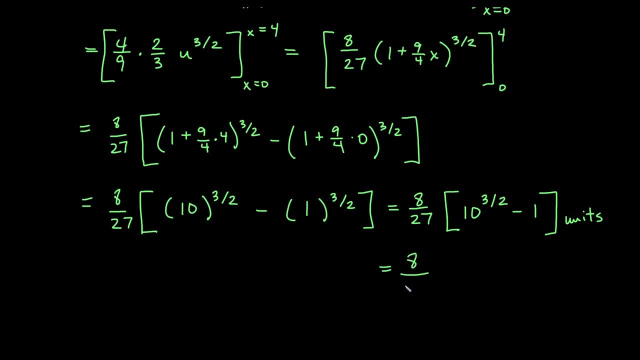 terms of roots. so you may see somebody who does a problem similar to this might say so this would be the square root of 10, and then cubed right. so you might have something like the square root of 10 cubed inside the brackets here minus one, and then they may simplify it further and they may go ahead. 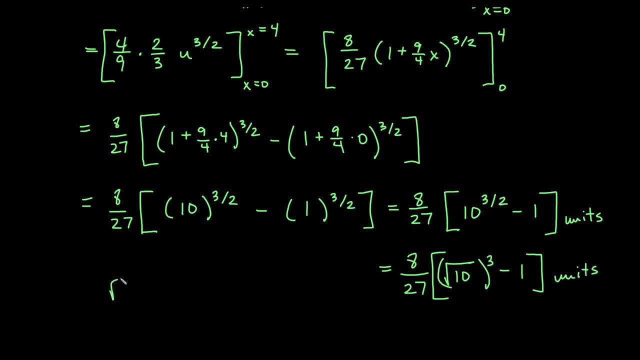 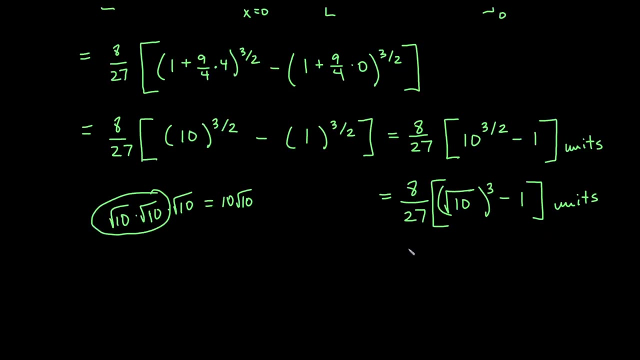 and see three copies of a square root right. so if you think about root 10 times root 10, two of those copies makes a 10 right? so this would really be 10 root 10, and so what you may see as a final answer from a lot of people on this one would be something like 8 over 27 in the front. 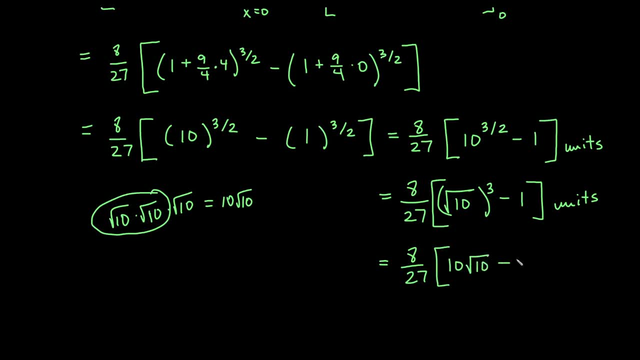 and then they would say 10 root 10 minus 1 and its length, which is one dimensional quantity, so we would say units there. okay, hopefully this helped With a similar problem you might be working on or just your first attempt at doing one of these check. 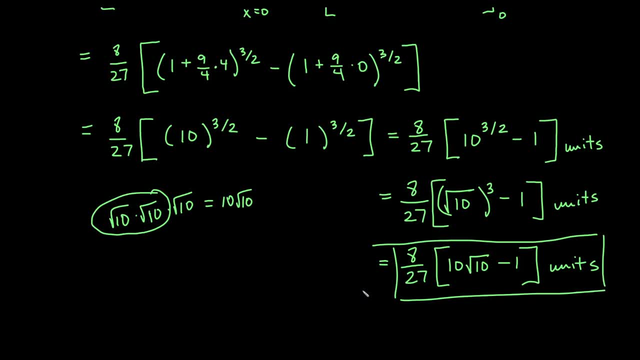 out the next example videos. they involve a little bit more creative factoring and doing some of these problems.